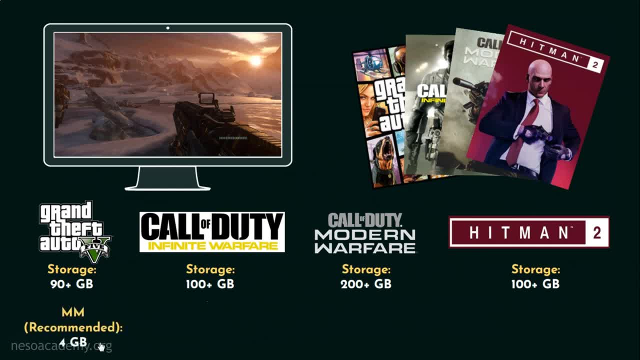 requirement for GTA 5 is only 4GB, For COD Infinite and Modern Warfare it's only 8GB, And for Hitman 2, it's 16.. Now, why so? It's because our operating system provides us with the concept of virtual memory and demand paging While playing. 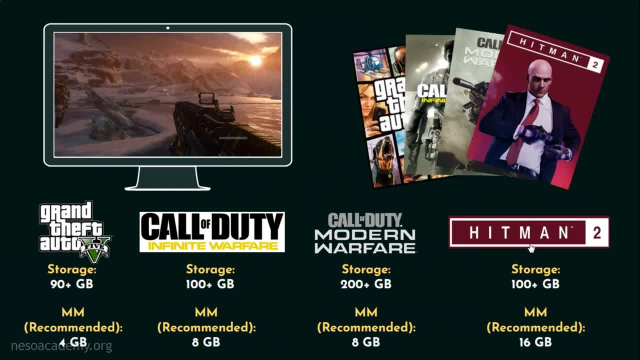 these or, technically speaking, while our processors are executing the codes of these games, they don't really require the entire 100GB code at once, And that's the beauty of it. That's why, having a way smaller main memory, we can still play the games without facing any. 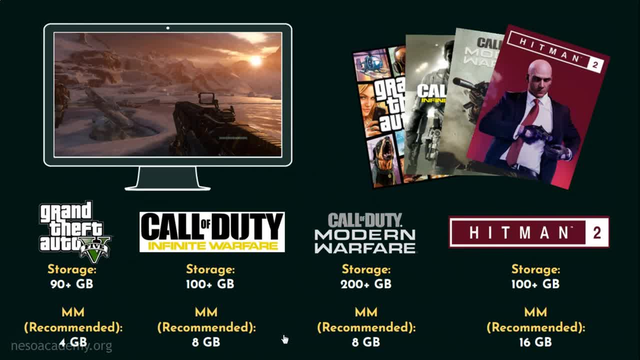 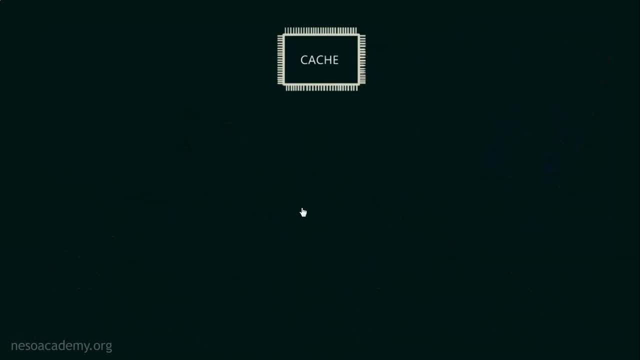 problems whatsoever, And just for the sake of understanding this concept in simple manner, we took the example of the code segment of just 100 instructions. Now let's talk about the cache. Again for the sake of understanding, I mentioned about cache memory as a single unit in our previous discussions. But to be precise, modern day. 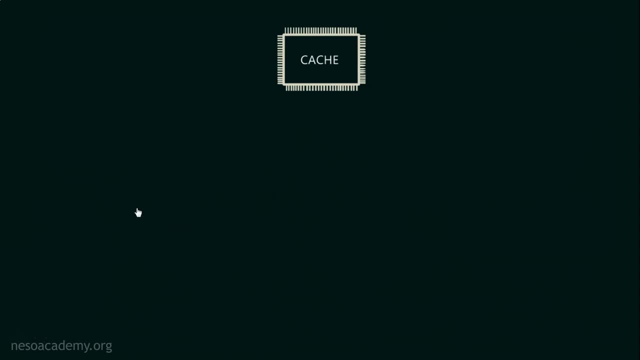 systems have levels of cache memories. Generally, there are three levels of cache used mostly in today's system architectures: The L1, L2, and the L3 cache. Now, as we have multi-core processors in our machines nowadays- you probably have heard the terms dual, quad, octa-core- Let me 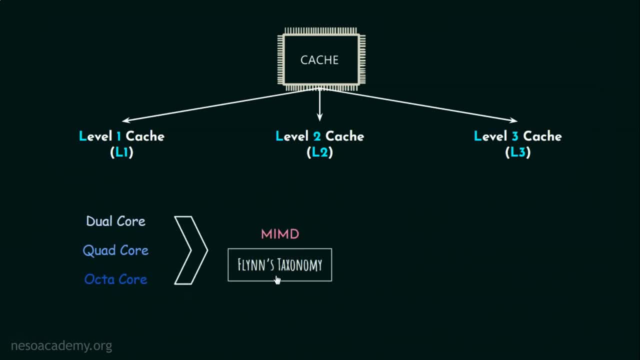 tell you these belong to the MIMD family of Flynn's taxonomy. I hope you remember that from our computer architecture classifications discussion. Now, L1 cache is embedded in the processor itself right from the days of its origin. Later, when the L2 caches emerged, 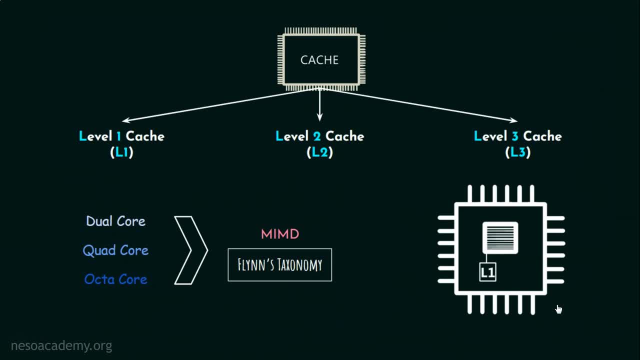 they were incorporated in the motherboard in their initial days, But now they are also a part of the processor itself. To be precise, different cores of the processors have their own L1 and L2 caches. Now coming to the L3 caches, they are also. 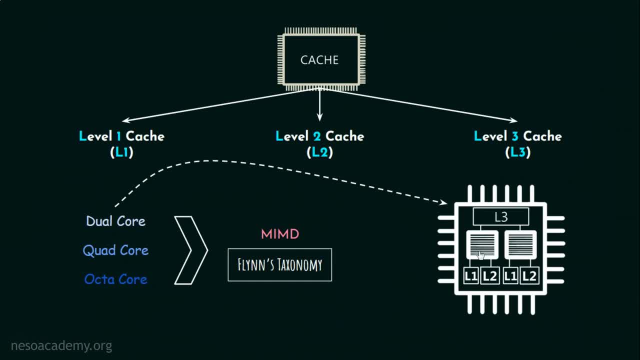 implanted in the processor, yet shared by all the different cores of the processor. By now you probably have the idea about these levels. Size-wise, L1 is the smallest, yet it is the fastest among all the other caches. L2 caches come after L1, and these are used. to store the L1, L2 caches go to L2,, and L2 contains all the letter L, So the L1 cache here is only three, though, or more than the other caches are only the EyeCook and the. 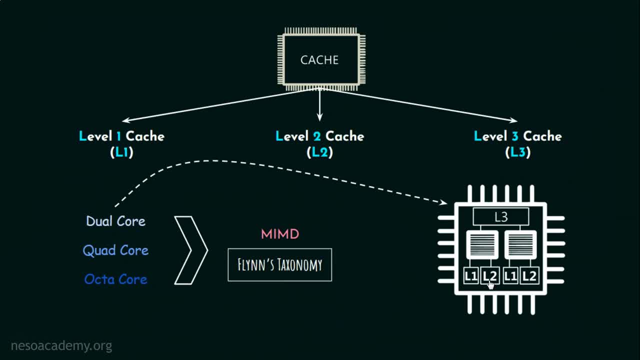 You INC partiable can identify from here and also is New Scot of the lots. In fact, many people stored the frequently accessed data which are second in priority. also, frankly, can't really be incorporated within the L1 cache due to the limitation of space. 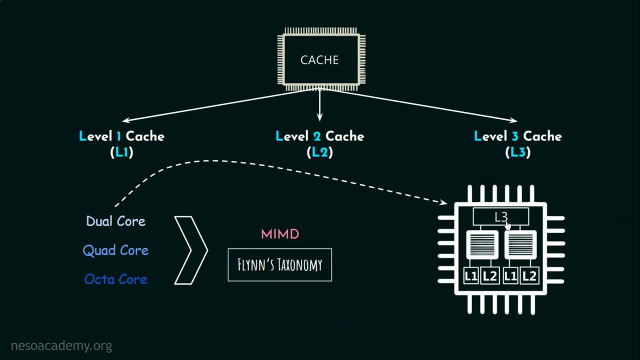 Finally, the L3 caches are the largest of all, and these are also called shared cache. Now, I hope the idea of different cache levels are clear to you In our later discussions. for the sake of simplicity, we will assume to have only a. 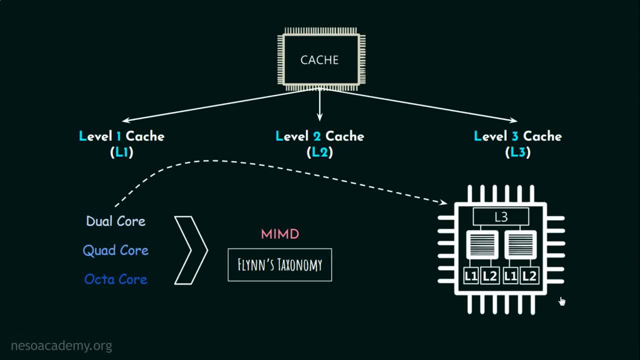 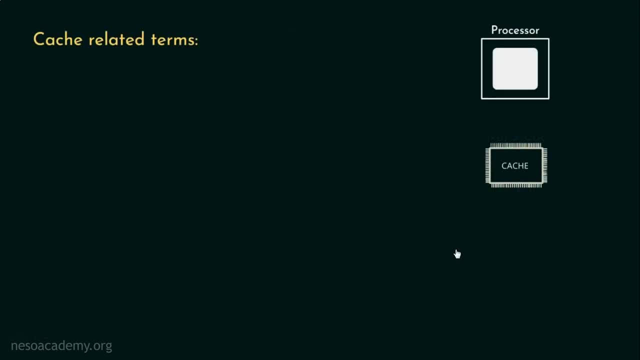 single cache mostly. However, I will provide detailed illustration of the various levels during the explanations of cache-level related numerical problems. Now let's get to know about a few terminologies related to cache. The first one: cache hit During execution if the processor is able to find out the required information in the 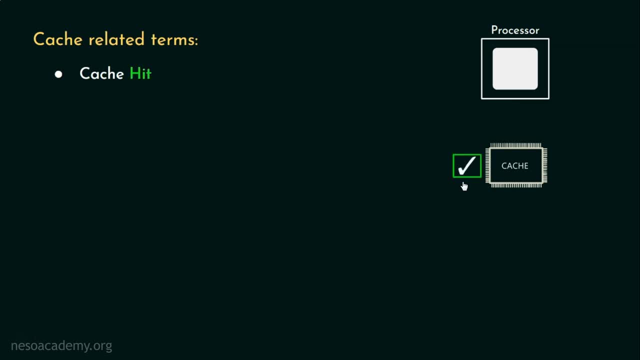 cache. we call it a cache hit, And the time required by this process is known as hit latency. Here, using a specific data structure called tag directory, the processor finds out whether the required information is present in the cache or not. Now, if the information is absent from the cache, that is, if the info is missing from 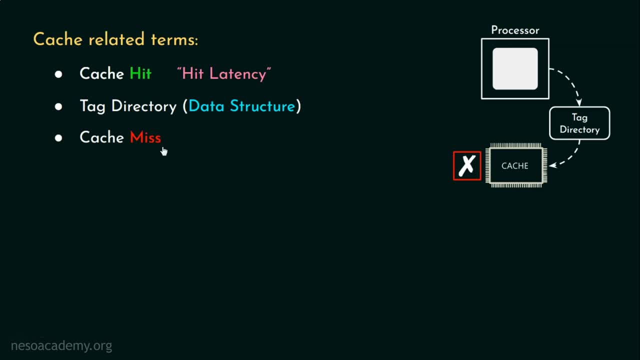 the cache. we call it cache miss. In this case, as discussed earlier, the processor will seek for the information in the next level of memory, which is the main memory, and bring it from there also, meanwhile, place it in the cache itself. 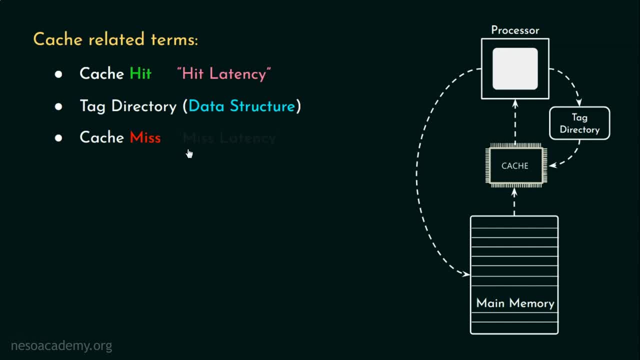 This entire period of time is called cache miss And FYI. if the information is absent, also from the main memory, the situation is called page fault And if found we call it page hit During page fault. the OS, as it, manages all the intercommunication between the main memory. 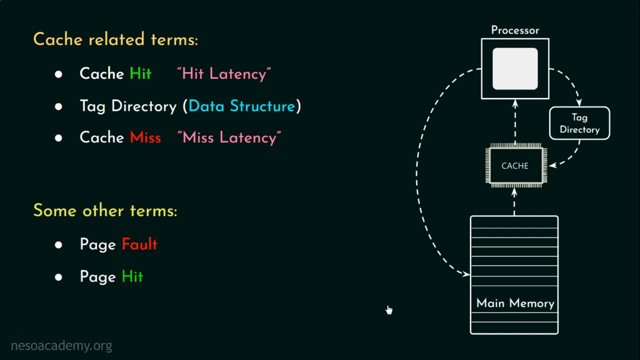 and secondary memory looks for the information in the last level of the hierarchy, that is, the secondary storage, and brings it back in the main memory. This entire process is known as page fault service. Thus the time taken to perform it is termed as page fault service time. 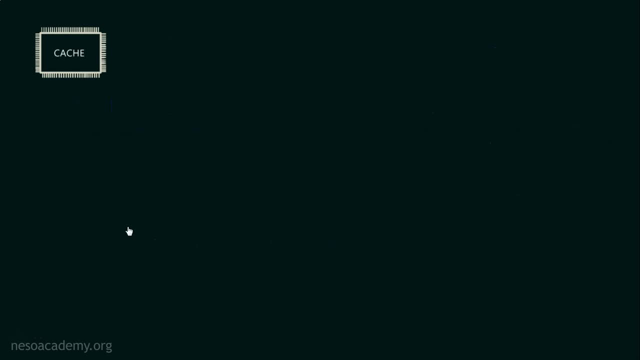 Now we already know that the information whose requirement frequency is very much higher than the others are generally kept in the cache. Now, this prioritizing of the parts of the main memory which are to be loaded inside the cache is done using the locality of reference.